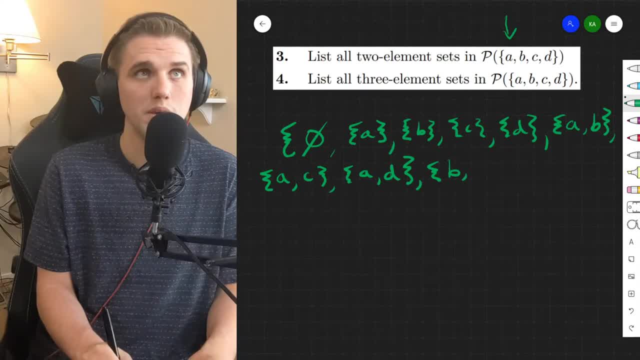 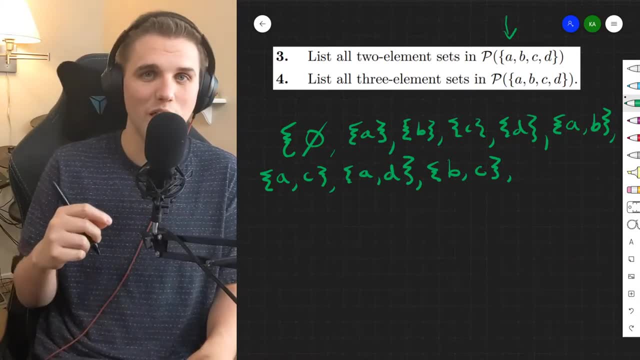 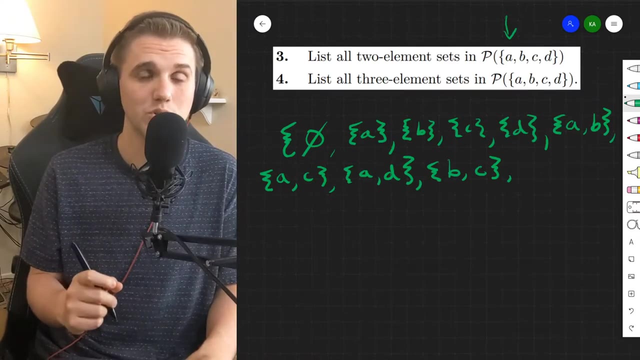 So we skip that B and A and we go straight to B and C. We can't do B and B because we can't pull out the element B twice. We can only pull out the element B once And again with every set. you can only have at most one object in that set. 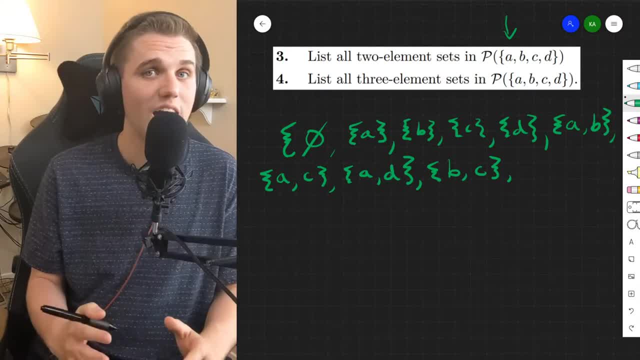 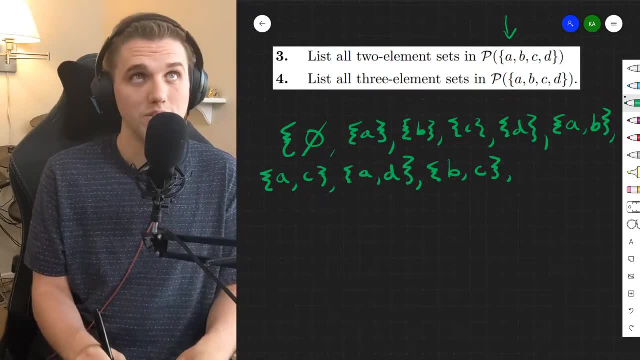 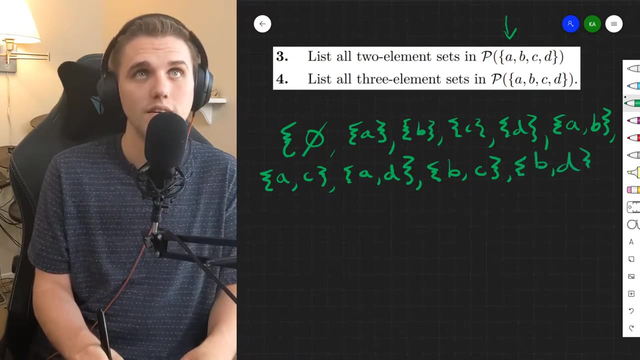 That is, And keep in mind that with a set, you can only have one copy of every element. You can't have more than one copy of any element. That would be a multi-set. All right, let's keep going. We have B and D and then C and D. 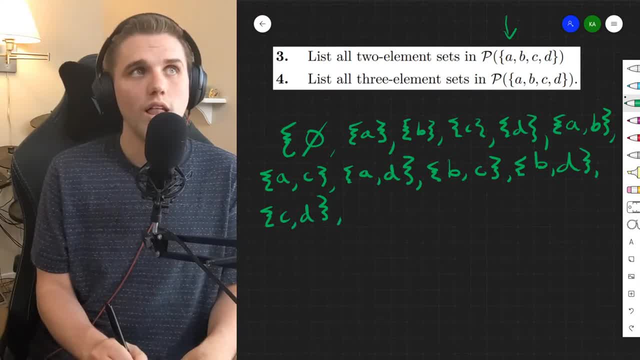 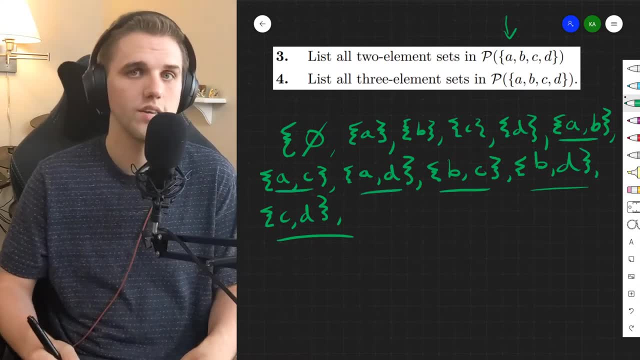 So this is the set. So how many two-element subsets do we have? We have 1,, 2,, 3,, 4,, 5, 6.. So the answer to problem 3 is 6.. But why is it 6?? 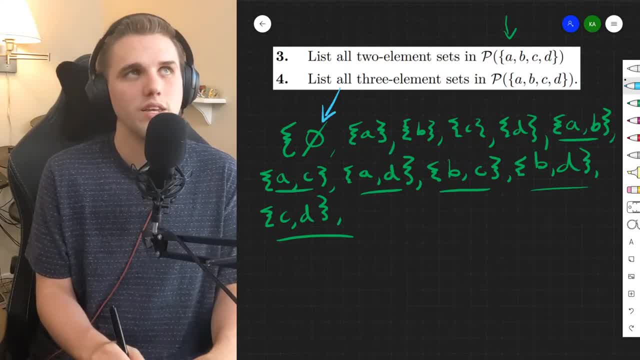 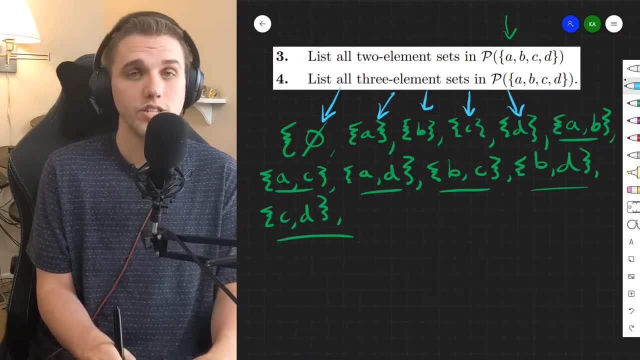 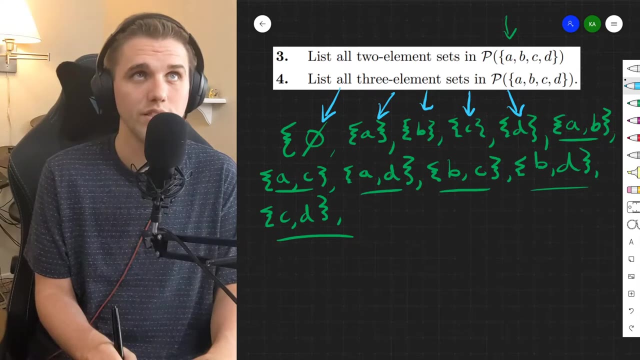 So I have a question for you all: Why is there an element here that is a set with zero elements? Why are there 4?? Why are there 4 sets here, or subsets, I should say, that are singleton sets, meaning that they only have one element in those sets. 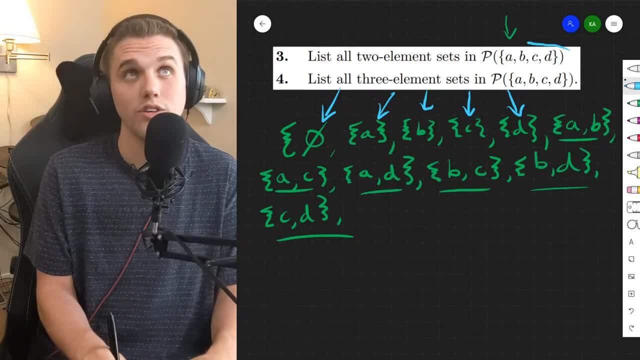 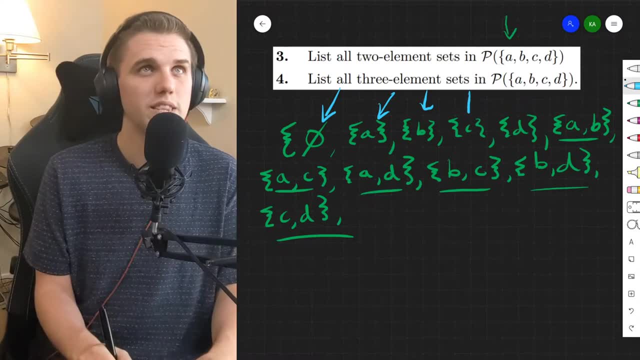 Why 4?? That's an oddly specific number. Well, it just so happens that there are 4 elements in my original set. Keep that in mind. That's important. But then how many sets, or subsets I should say, have 2 elements? 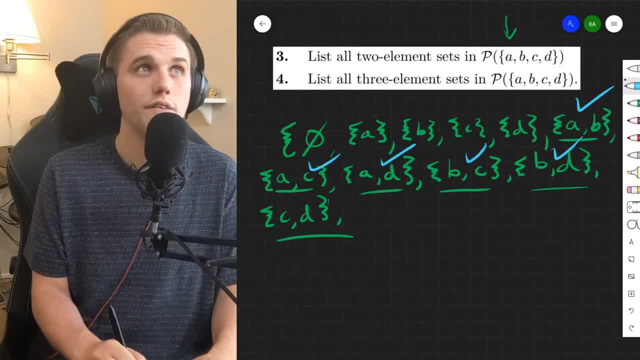 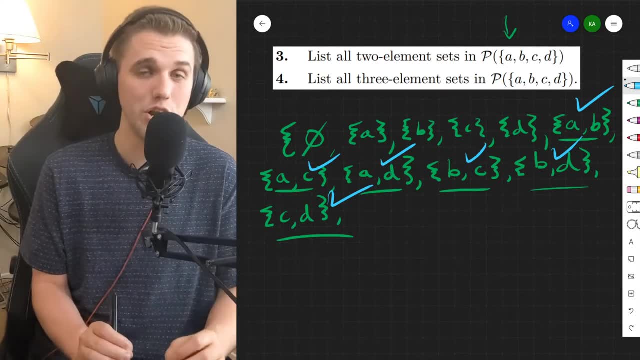 Well, we said 6.. 1,, 2,, 3,, 4.. 5,, 6.. But why 6?? Where does 6 come from? Well, we'll actually address this specific question multiple times throughout Discrete Math. 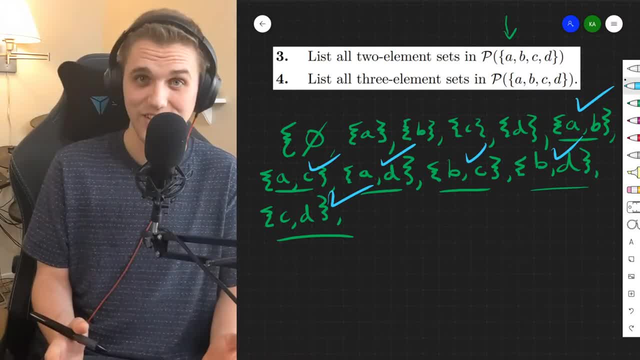 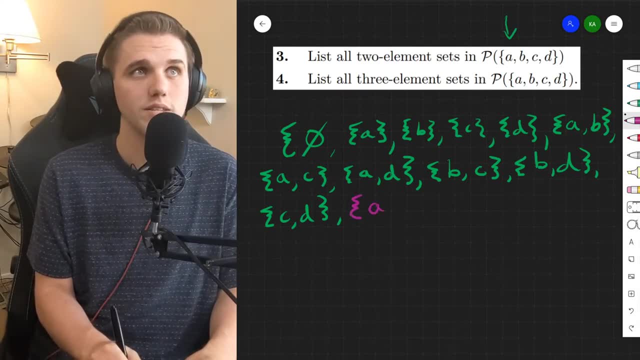 But for now, just know that the answer is 6, because that's what we counted. What about the sets with 3 elements, or the subsets, I should say, of 3 elements? Well, we could do A, B and C. 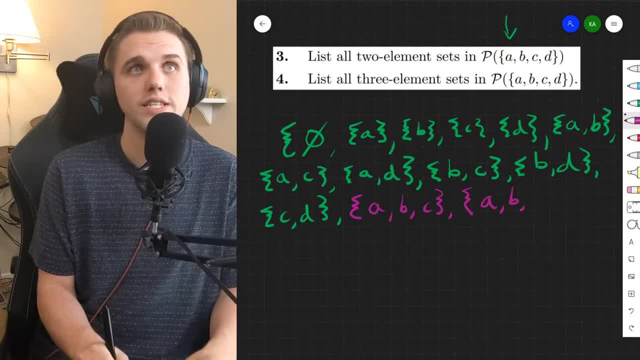 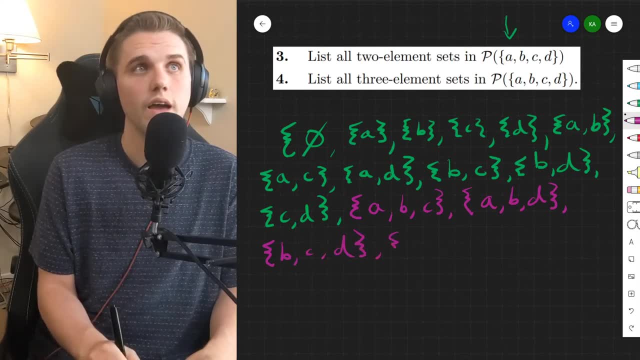 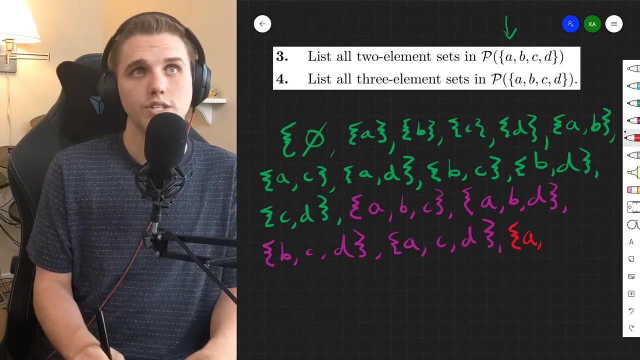 We could do A, B and D. We can do. We can do B, C and D and A, C and D. And then, last but not least, in our power set, we have a set of size 4, which is A, B, C and D.